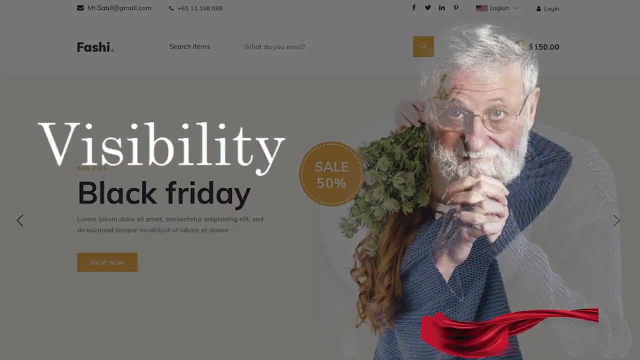 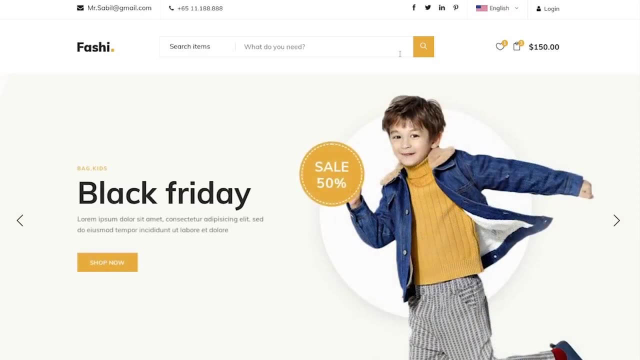 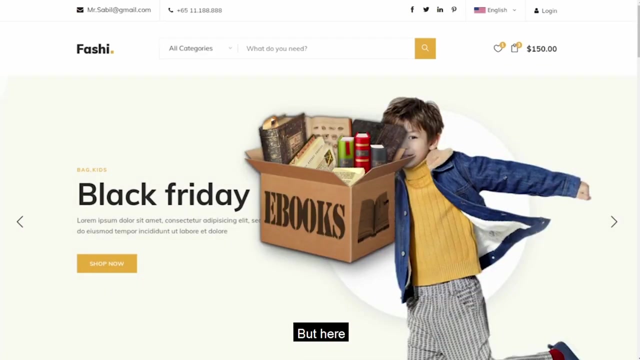 options are and know straight away how to access all of them. This is a good looking e-commerce website, But the only function you get is Search items. In e-commerce, there should at least be categories, options, price range and a card value, but here there are no such options available in. 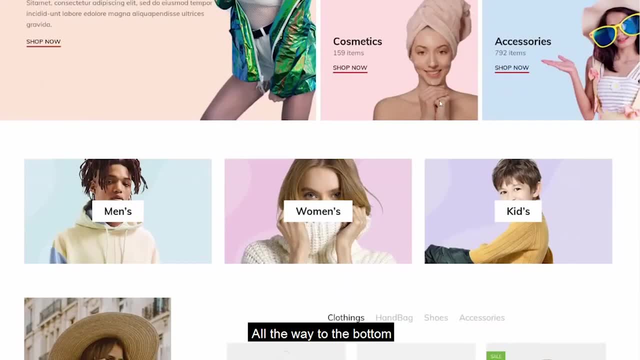 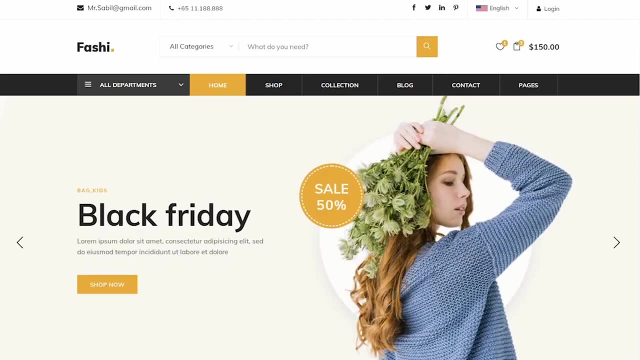 the beginning. User must scroll all the way to the bottom to find the options. Now let's redesign the website to get the visibility. This is the redesigned website. Here all the options are displayed in the letter Welcome. There is a link to tutorials. 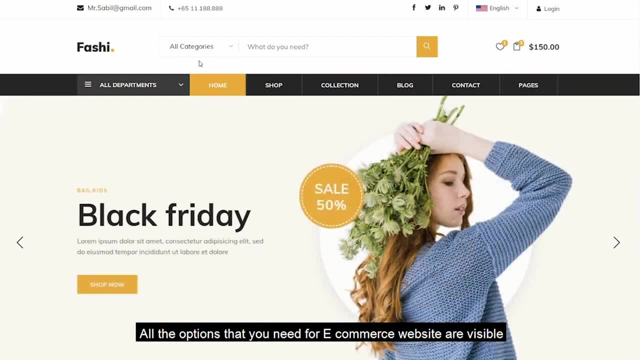 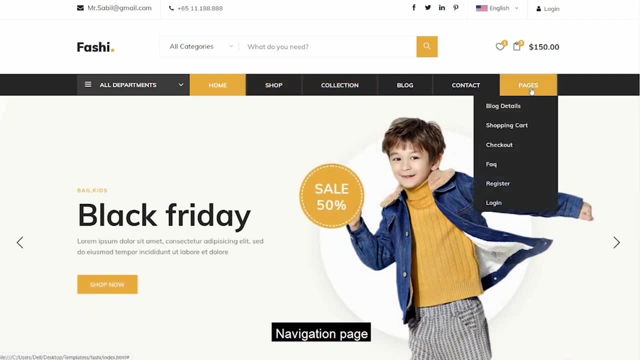 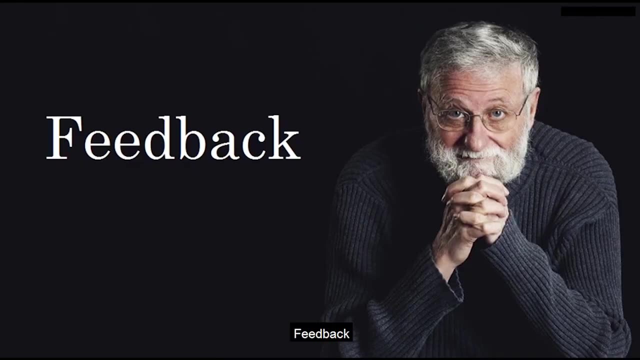 options that you need for our e-commerce website are visible. categories, option department, different section of cloth clothing- are available. navigation page and shop where you get range of pricing options in the left. feedback- feedback means reaction caused by action. there needs to be some indication, like sound, a. 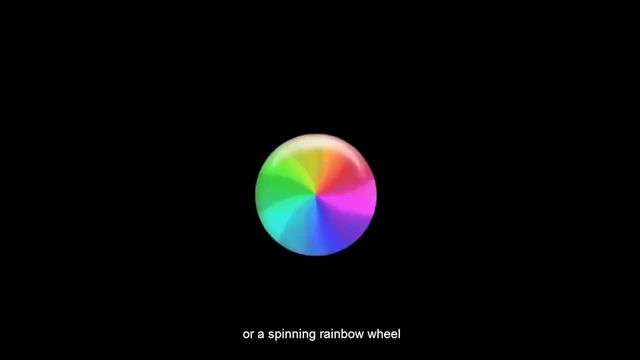 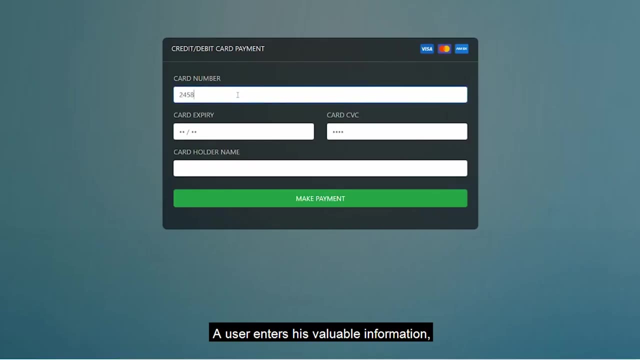 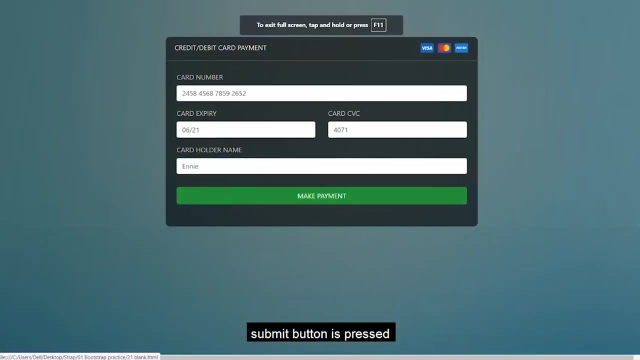 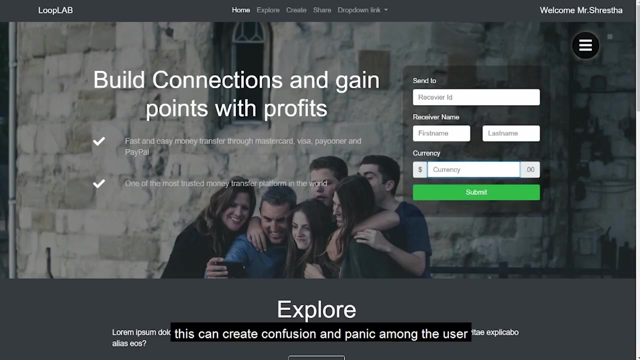 moving dial or a spinning rainbow wheel example. here in this payment website a user interest is valuable information, including his credit card number. for case one, submit button is pressed but without any action the website is redirected back. this can create confusion and panic among the users. he see cannot confirm if he's our payment was. 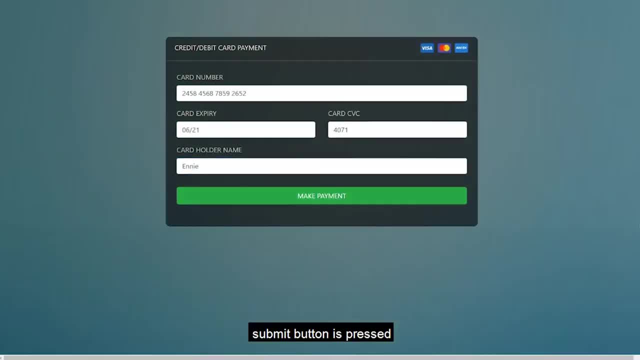 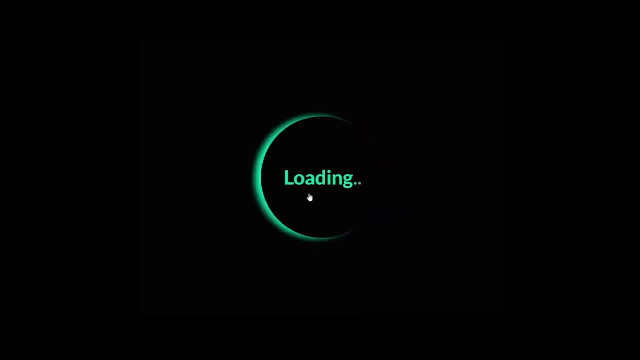 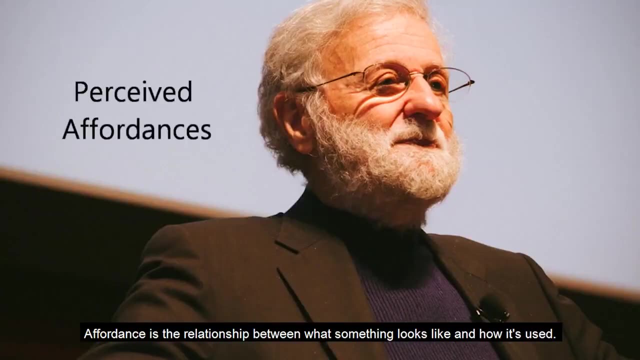 successful or not. for case two, submit button is pressed here. the loading icon is the feedback which asserts that the process of the transaction is going on. let's understand what is affidavit. affidavit is the relationship between what something looks like and how it is used. for designers, it means that as soon as 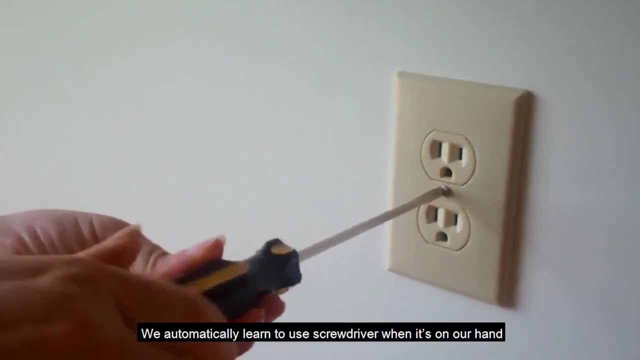 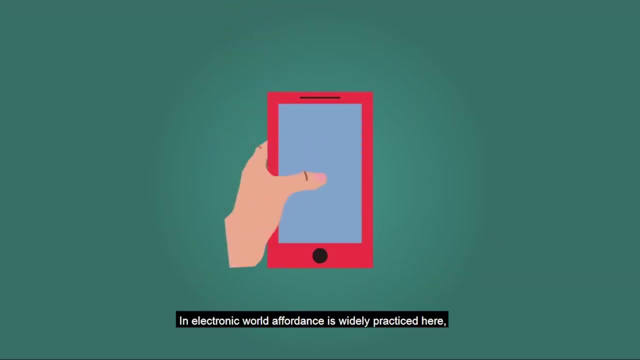 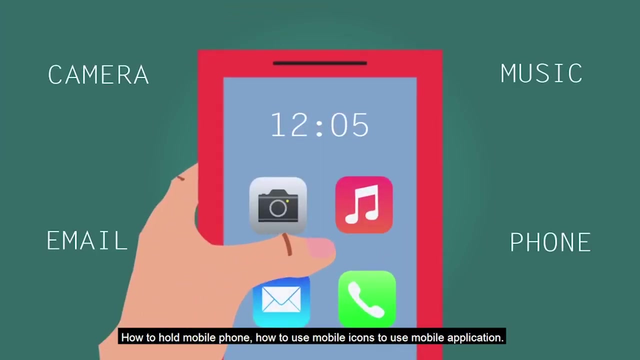 someone says something, they have to know how to use it. we automatically learn to use screwdriver when it's on our hand. in electronic world, evidence is widely practice here, while phone has higher fisherman's is to figuring independently how to use it: how to hold mobile phone or to use mobile. 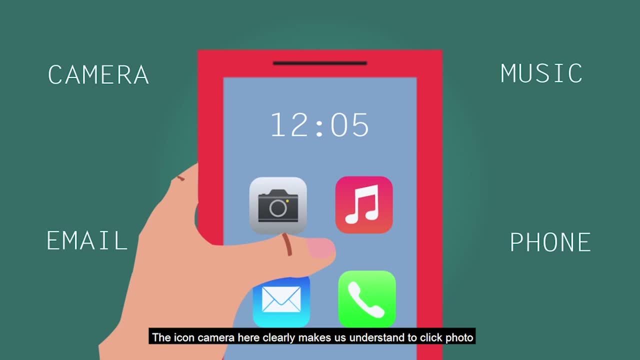 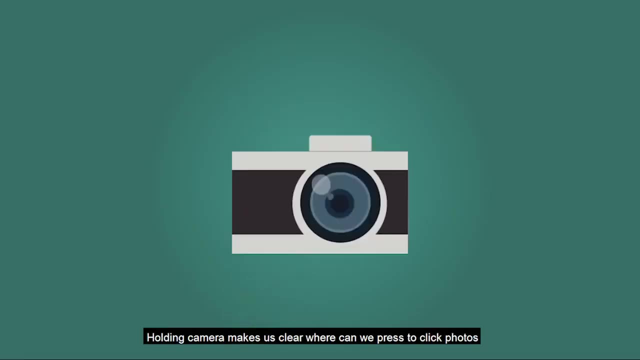 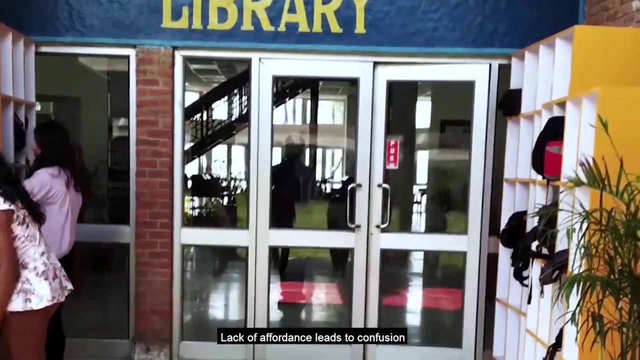 icons to use mobile application. I can camera here clearly makes us understand to click photos. similarly, messaging icon for sending messages and so on, holding camera makers clear where we can press to click photos- lack of evidence leads to confusion- are really confusing. mapping are used to determine relationship, typically between 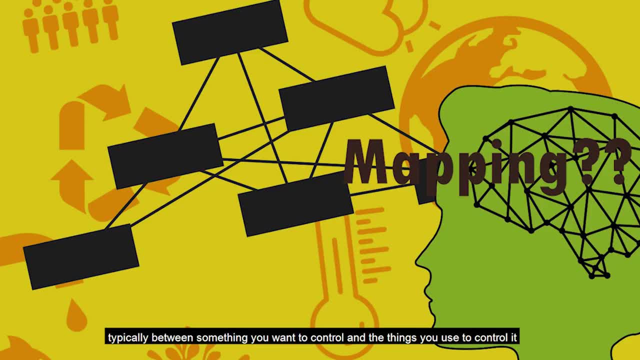 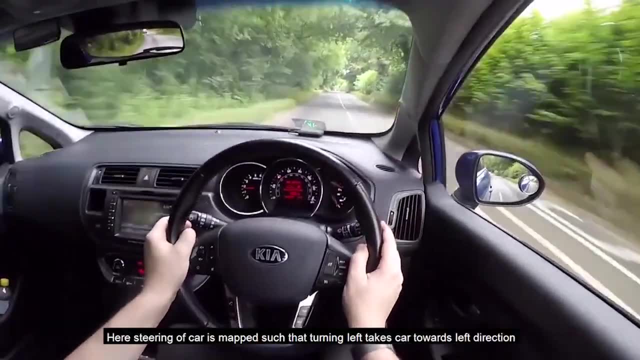 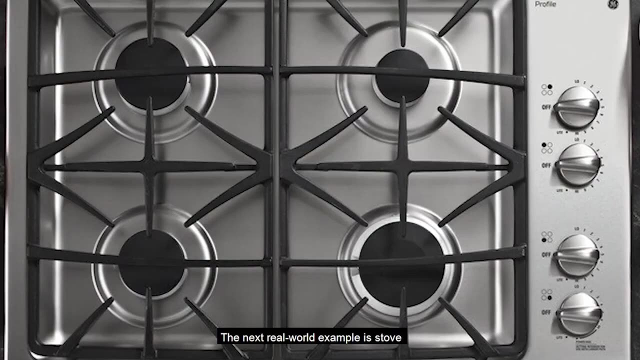 something you want to control and the things used to control it. let's go to quick example. here, steering of a car is mapped such that turning left takes car towards left direction. likewise, turning right makes car to drive right. the next real-world example is stop here the stop. it has four burners and there are four. 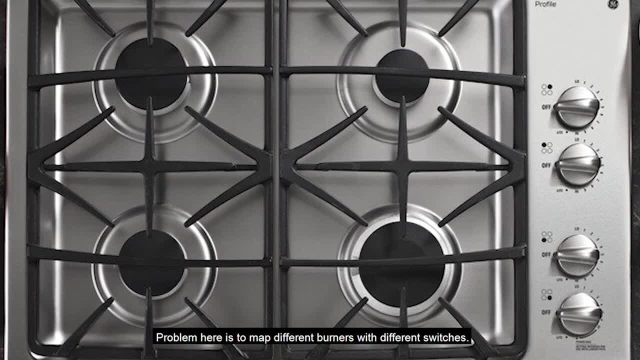 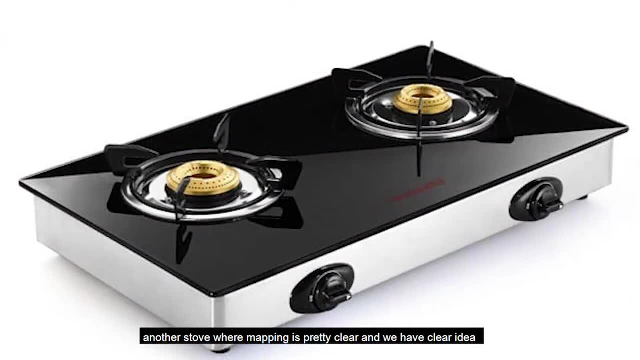 switches or dial to control four burners. problem here is to map different burner with different switches. so here another stop where mapping is pretty clear and we have clear idea which switch is used to control which burner. this is proper mapping constraints: constraints are the design features that limit the range of 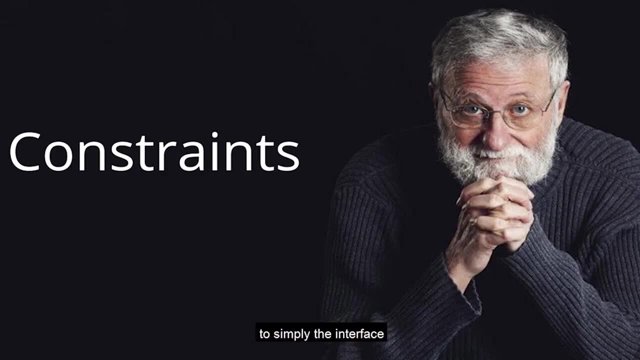 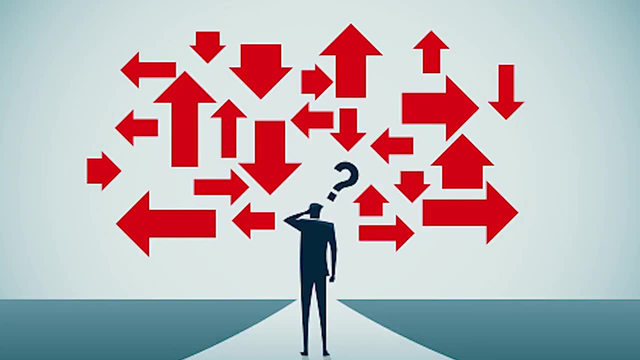 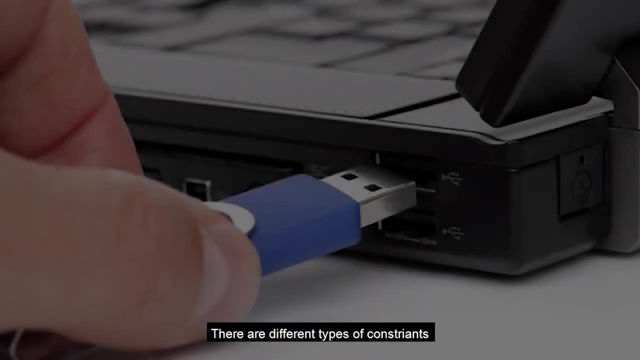 possible actions or interactions that user can take to simplify the interface and guide the user to appropriate next action. limitless possibilities often leave the user confused. constraints narrow down the set of options user have to consider, reduce the chances of error and make your task easier. there are different types of 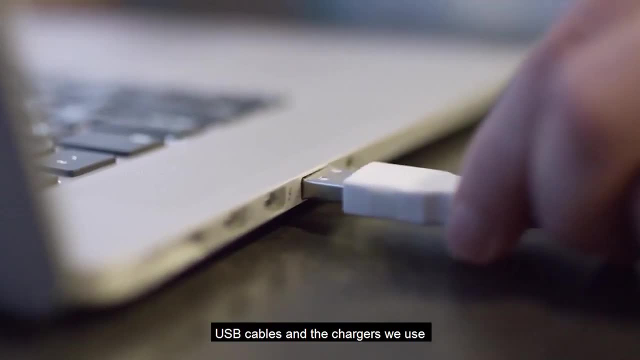 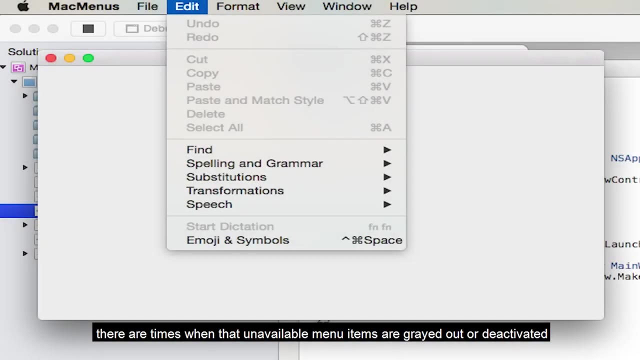 constraints, for example physical constraints, USB cables are the charges we use. some of these cables can only go in one way, not the other. and about illogical constraints. there are times when the unavailable menu items are read out or deactivated. for example, here on the Windows Explorer the paste option is. 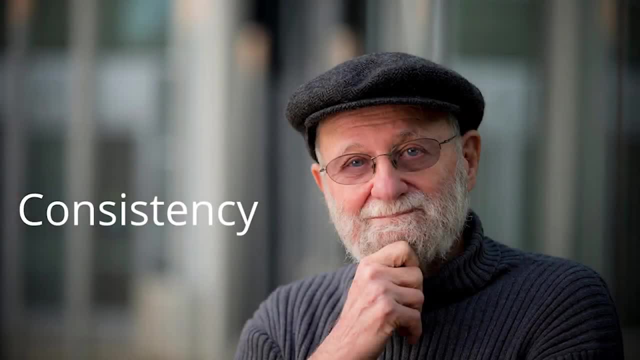 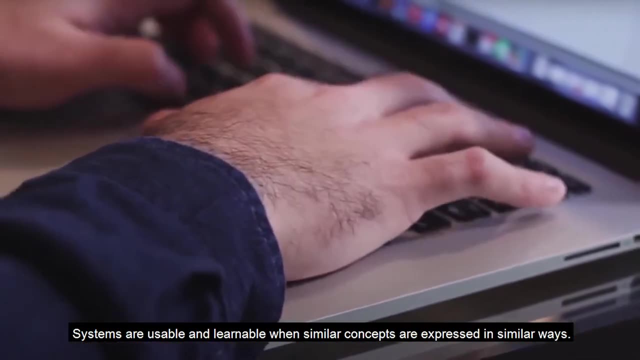 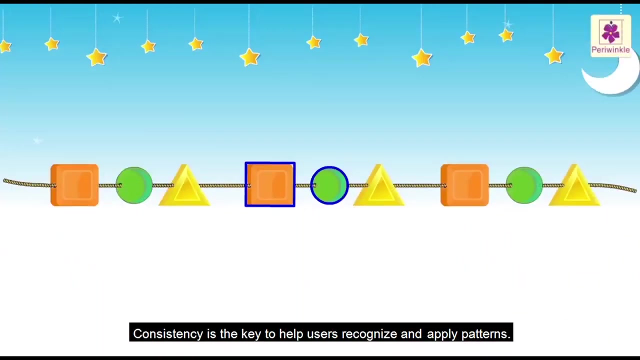 faded, as you can see here. it is not activated. and it is not going to be activated as it is unavailable. consistency: consistency refers to having similar operations and similar elements for achieving similar tasks. systems are usable and learnable when similar concepts are expressed in similar ways. one of the major ways that people learn is by discovering patterns. consistency: 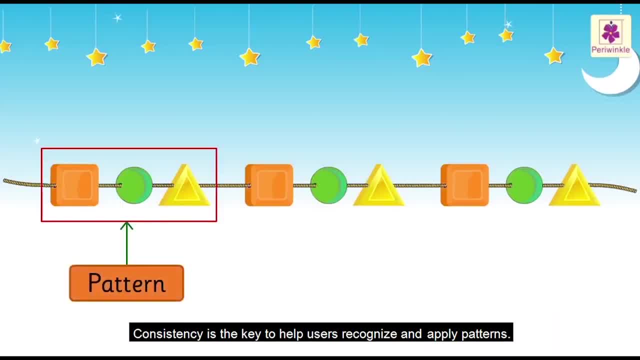 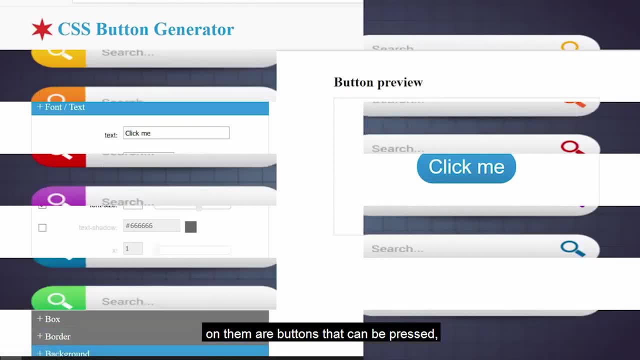 is a key to help users recognize and apply patterns. things that look similar should do similar things. for example, if you learn that protruding surfaces with labels on them are buttons that can be pressed, then the next time we see it we will tend to recognize it as a pressable button. inconsistency causes confusion.